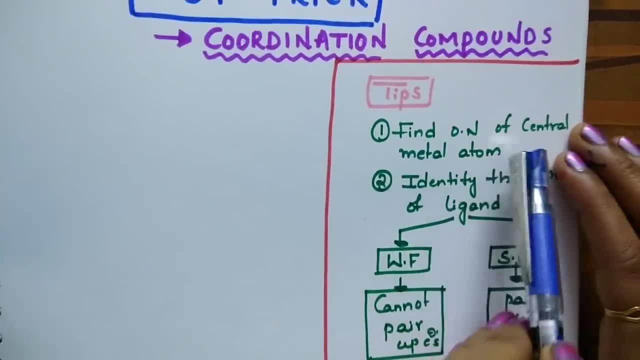 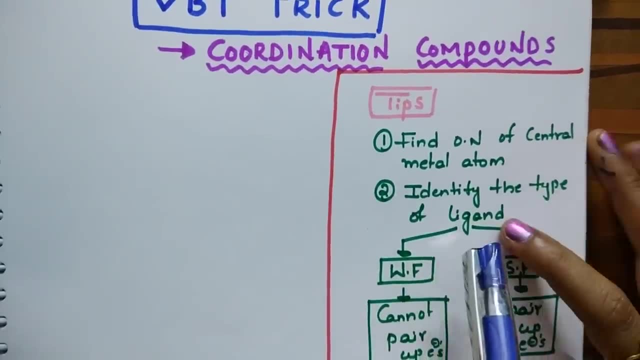 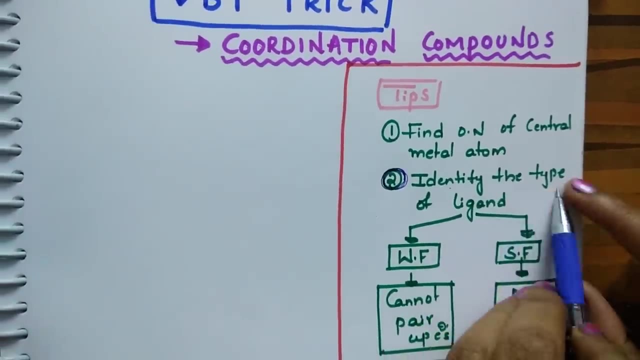 Tip number 1. Find oxidation number of the central metal atom First. what you have to do, You have to find the oxidation number. After finding oxidation number, just what you do is- this is the key step most important- Identify the type of ligand, Whether the ligand is a weak field ligand or strong field ligand. just identify that. 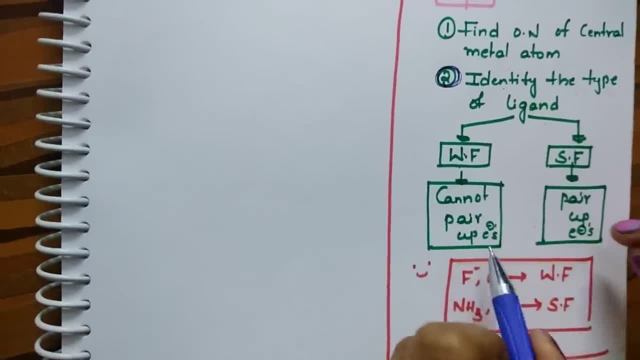 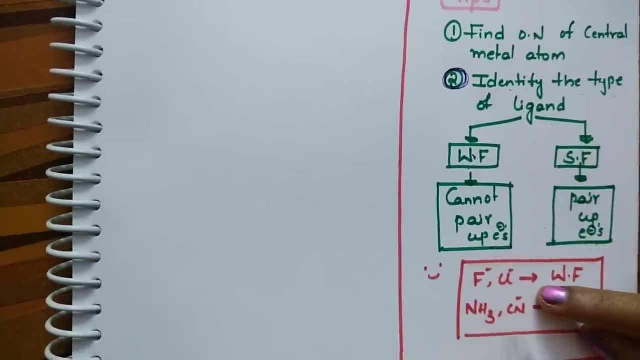 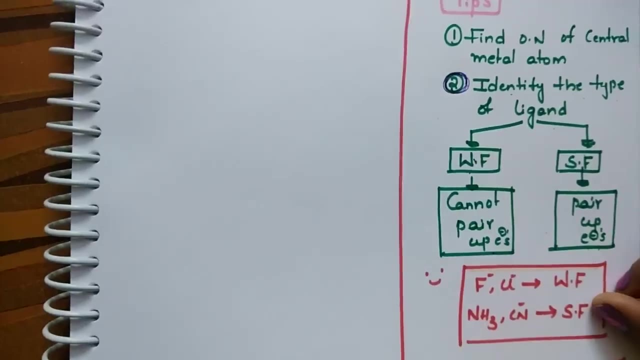 Suppose: if it is a weak field ligand it cannot pair up the electrons. If it is a strong field ligand, it pair up the electrons. Here by taking 4 MCRT examples I am giving this: F-Cl- are weak field ligands and He3 and Cn- are strong field ligands. 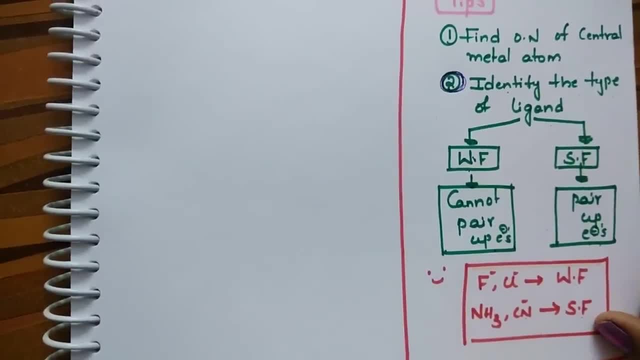 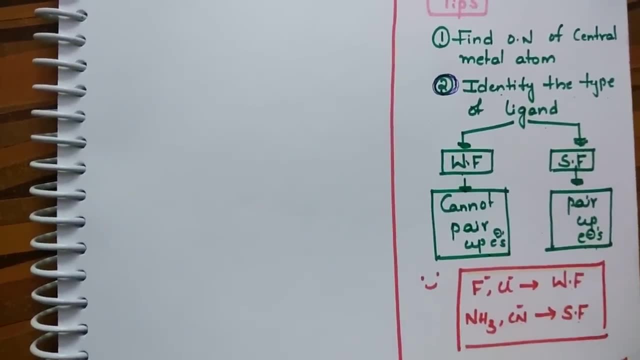 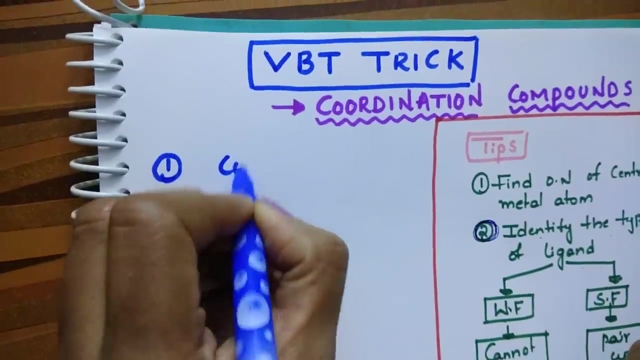 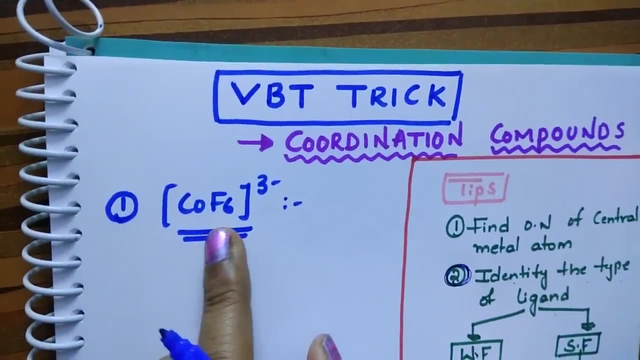 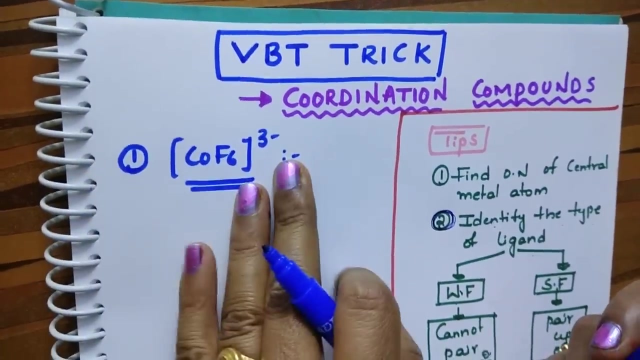 While you are doing with different examples, what you do is just follow the spectrochemical series to identify whether the ligand is a weak field ligand or strong field ligand. Let's start Tip number 2.. Find its hybridization, find its magnetic nature, find its whether it is an outer orbital complex or inner orbital complex by using this VBT. 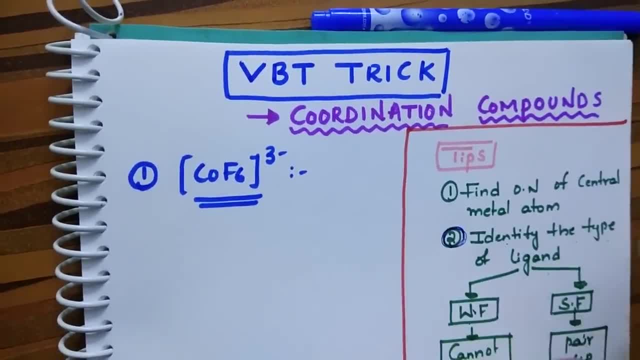 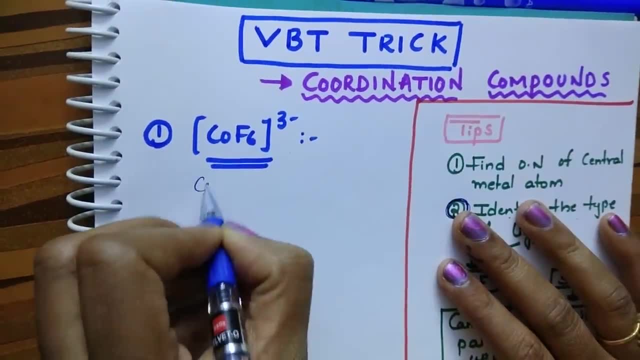 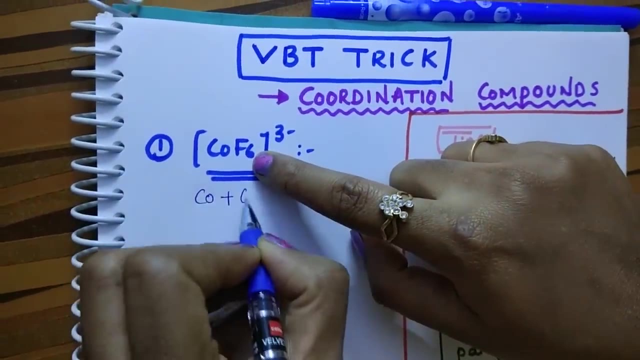 That is your question, Tip number 3.. Tip number 4.. Find its oxidation number, CO+. We know that the sum of the oxidation numbers- see here, 6 are there right. 6 into F is equal to minus 3, is equal to its charge, right. 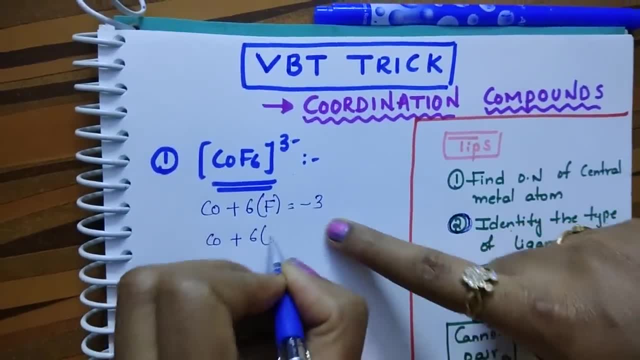 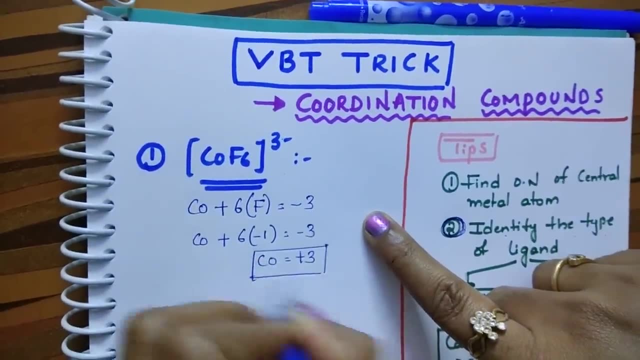 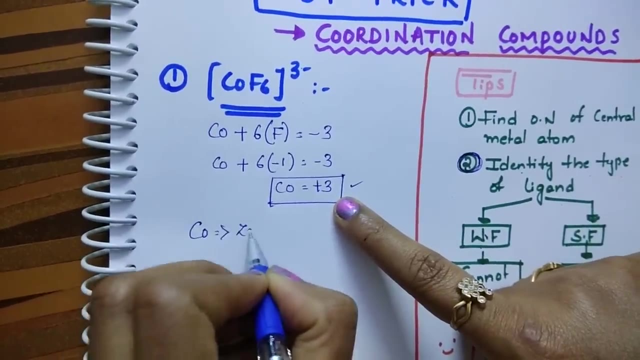 CO plus each fluoride ion oxidation number is minus 1, which is equal to minus 3.. Then cobalt is equal to plus 3.. What is the oxidation number, student? Cobalt oxidation number is plus 3.. What you do is cobalt atomic number is 27,, right? 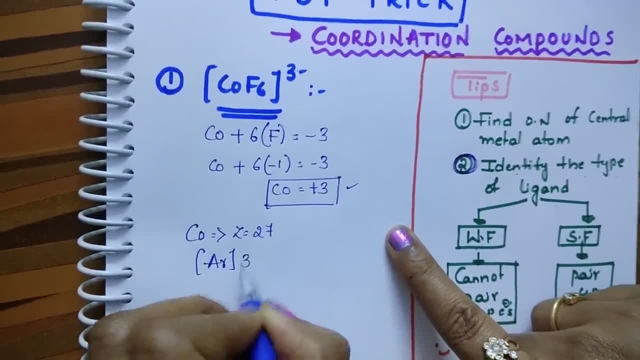 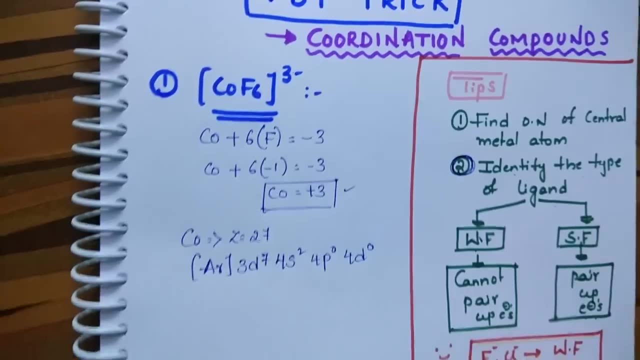 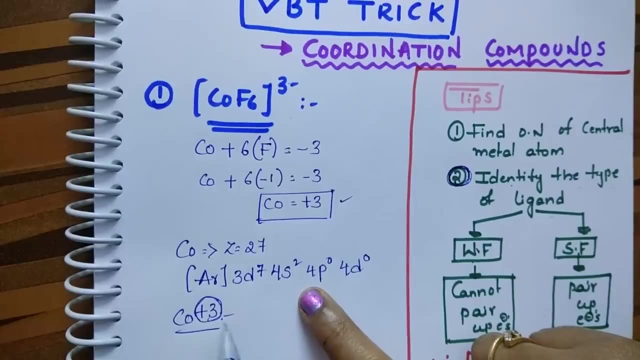 Its electronic configuration. argon 3D is 7,, 4 is 2.. 4P also will be present, but no electrons. 4D, there will be no electrons right? What you do is cobalt. it is present in plus 3 oxidation state. so remove 3 electrons. 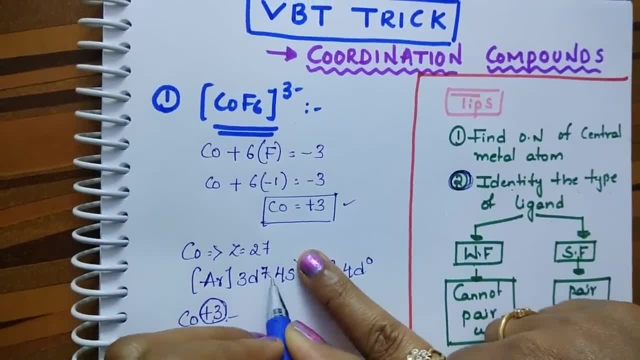 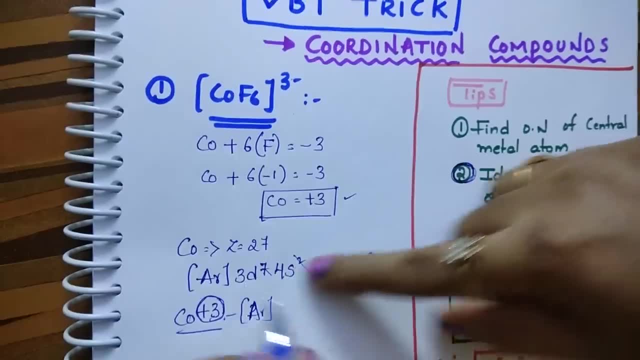 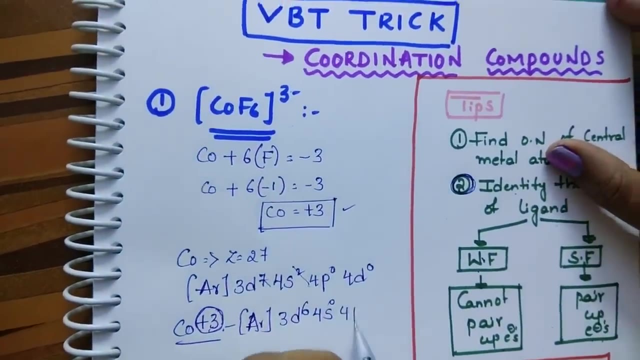 It is in plus 3, remove 3 electrons, 2 from S, 1 from P, So it will be Argon first remove from S, then D, argon 3D 6, 4S 0, 4P 0 and 4D 0.. 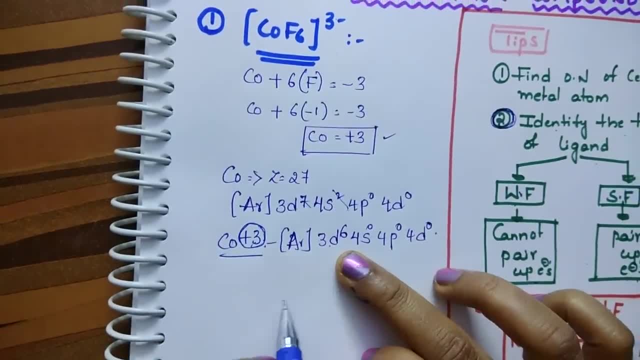 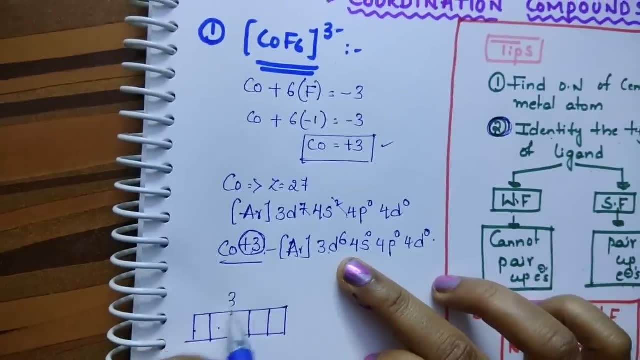 Then what you do is write the D orbital 3D. orbital D has 5 orbits: 1, 2, 3, 4, 5.. This is 3D, 6 and 4S. 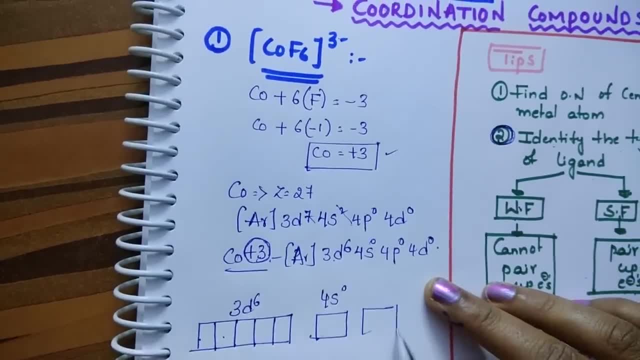 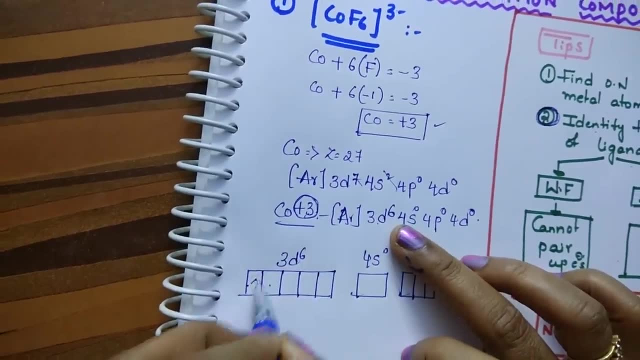 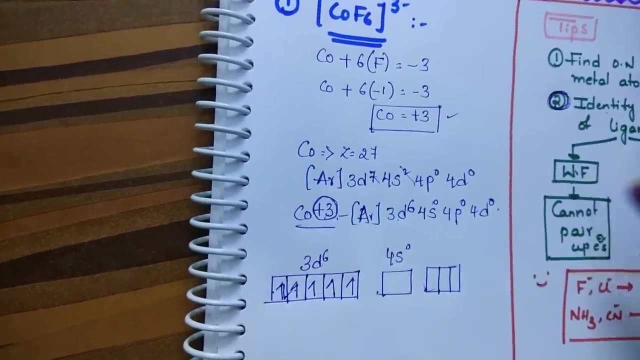 This is 4S 0,, next to 4P, and D also will be present. 5D orbitals will be there right. D is 6.. How many electrons are there? 6, 1,, 2,, 3,, 4,, 5,, 6? and here the thing is. after doing this, this is same for any complex 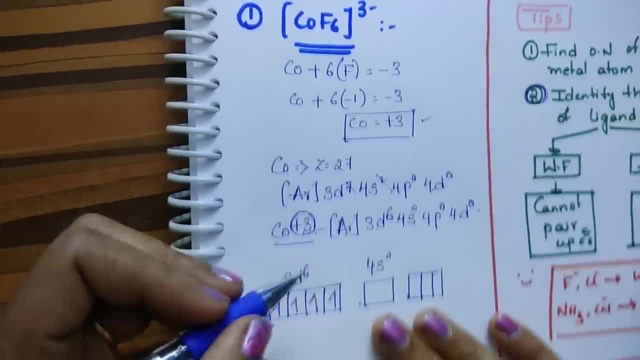 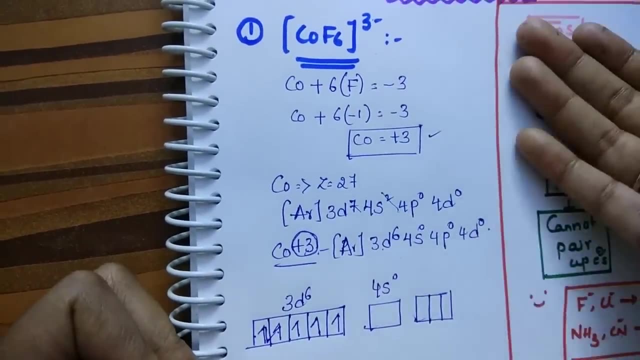 Whatever complex you take, this procedure is up to here. it is same. Is it clear Whether it is COF6, 3 minus or NiCN4, 2 minus, whatever the complex you take up to here, it will be same. 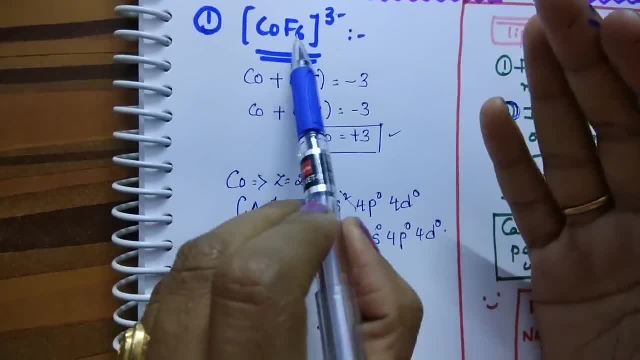 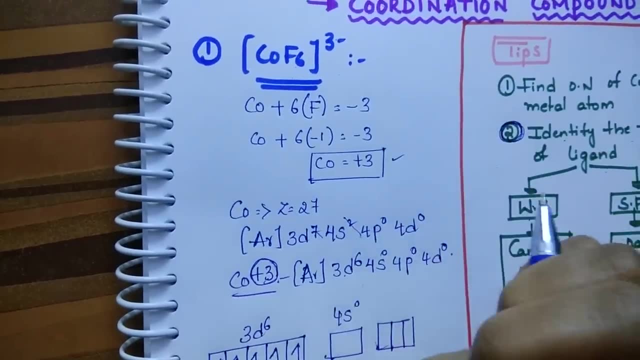 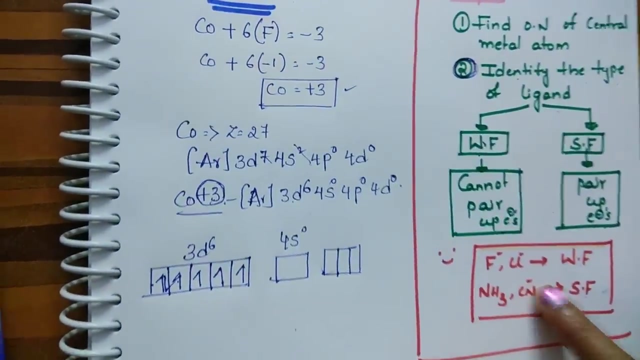 Now main part. whether this ligand is a weak field ligand or strong field ligand, identify it according to the spectrochemical series Based upon NCRT. this tip I am giving you: flow: F minus, L minus weak field, and H3 and CN minus is strong field. 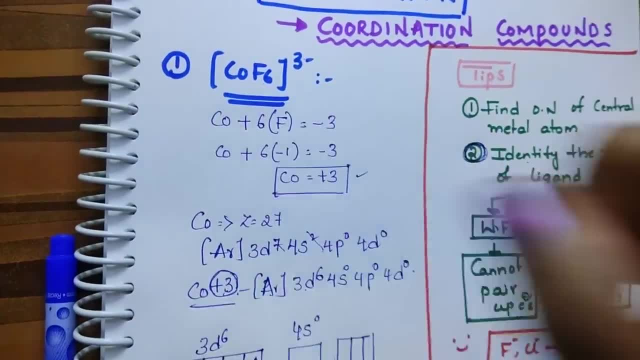 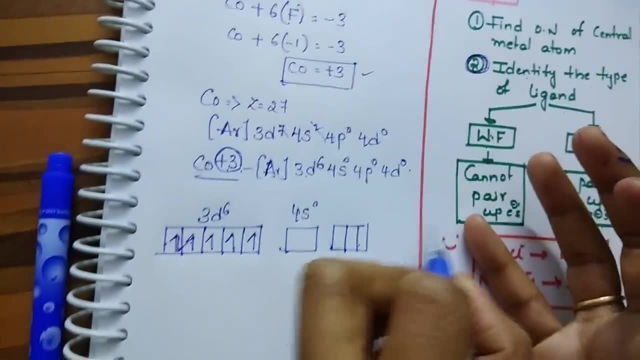 Here, F minus is Which ligand students? It is a weak field ligand so it cannot pair up the electrons. Then see here, Here it will be having 4S, 4P and even D also will be present, right? 5D orbitals. How many ligands are there? 6 ligands are there, So each ligand donate a pair of electrons. Each ligand donate a pair means each ligand requires one orbital, So what it do is. 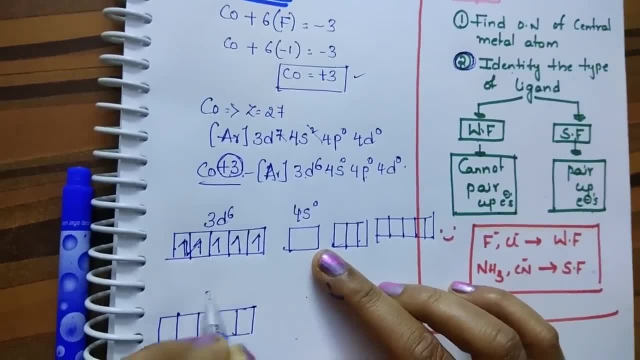 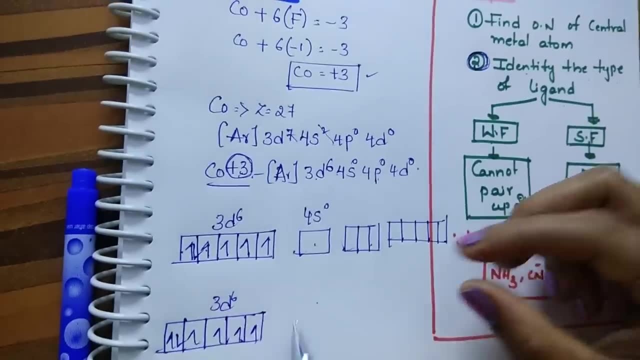 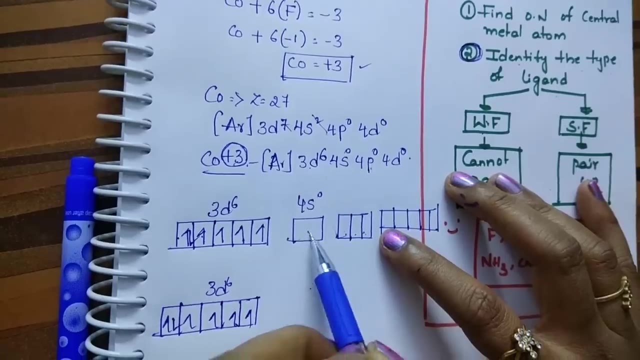 This is 3D6, 1,, 2,, 3,, 4,, 5,, 6 and each requires an orbit right. So total 6 orbits. it require 1, 2,, 3, 4, 1,, 2,, 3,, 4,, 5, 6 orbitals are there. 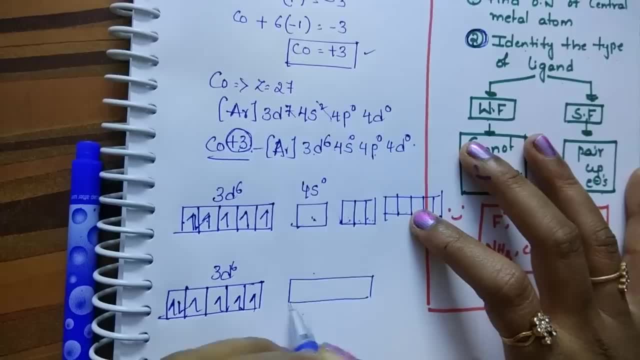 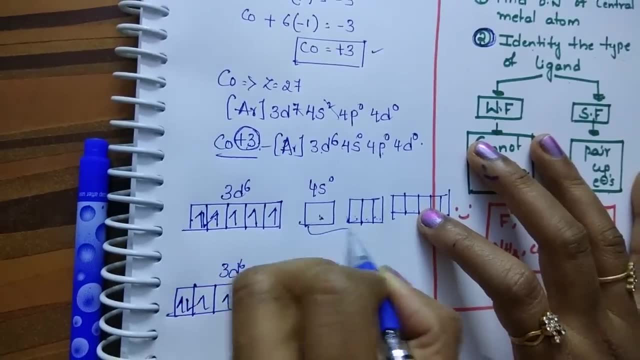 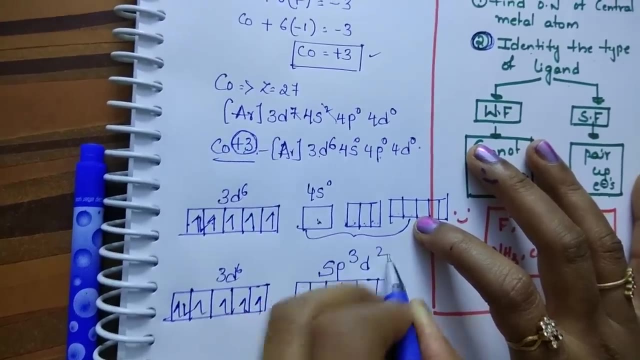 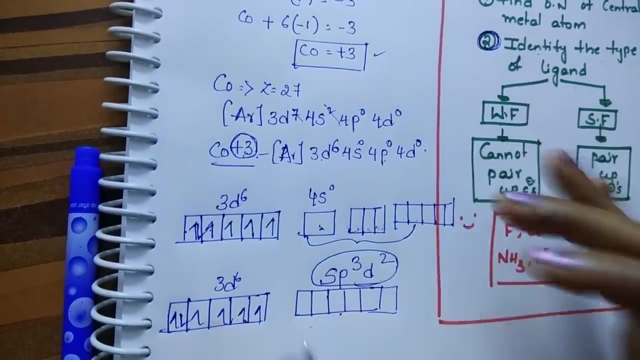 6 orbitals combine: 1,, 2,, 3,, 4,, 5,, 6. Means: 1S, 3Ps, 2Ds, 1S- 3Ps- 2Ds, So total the 6 orbitals overlap each other and it results in the formation of 6 hybrid orbitals. 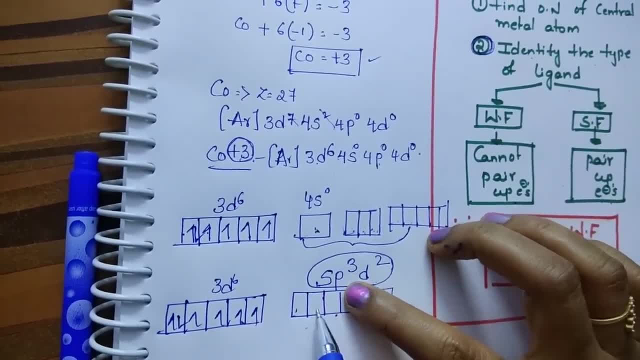 Each hybrid orbital: this is one SP3D2,, this is another SP3D2,, SP3D2, SP3D2,, like this, 6 orbit. This will be. this is what 4P right, 4P0, 4D0. 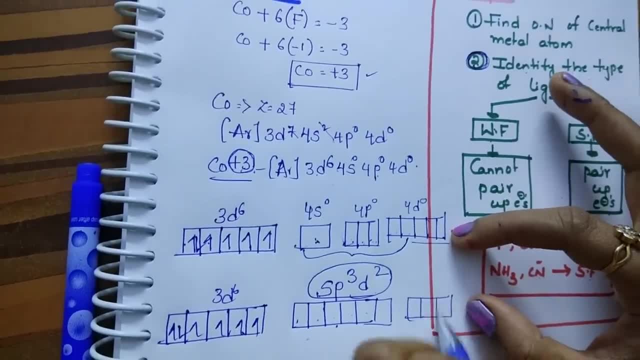 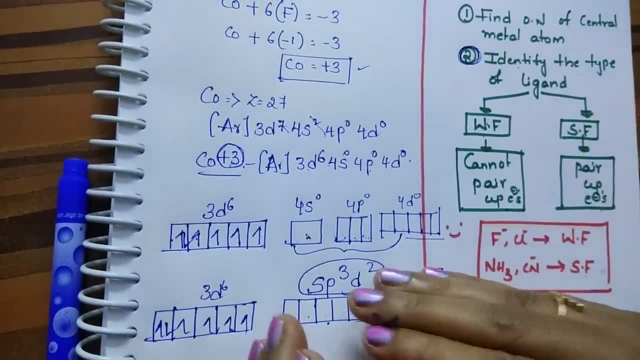 This is remaining. 3 are empty. This 3 are 4D orbitals are empty. right Now. this hybrid orbitals are present in the metal atom which are ready to accept electrons from the 6 fluorines, So each fluoride ion donates a pair of electrons. 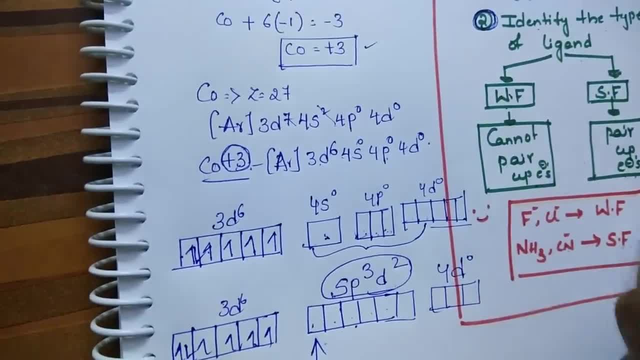 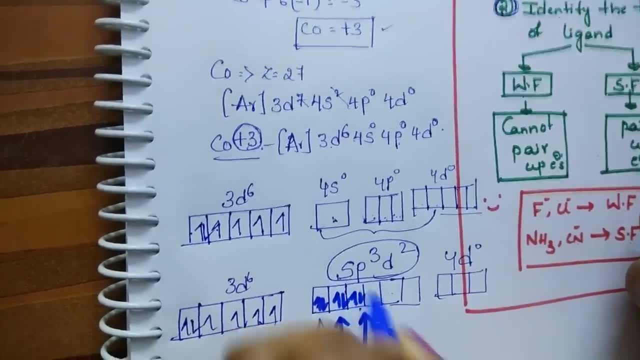 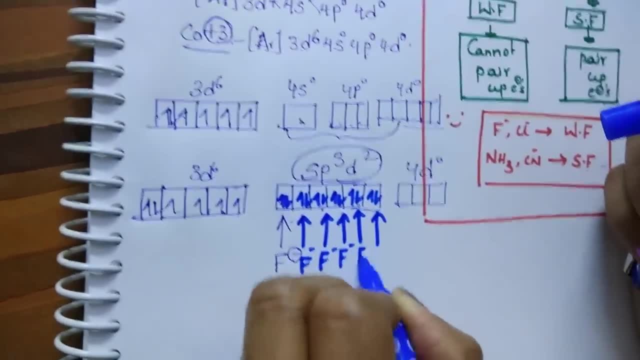 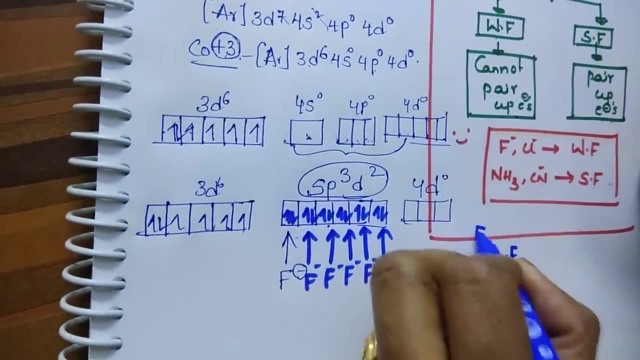 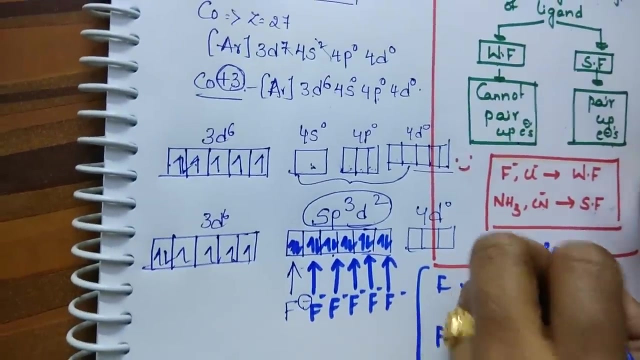 Means 6 fluoride ions donates a pair of electrons. each total 6 pair of electrons. it donates and it forms the complex with the metal. Right Now, your thing is: what is the hybridization? What is the hybridization, students here, 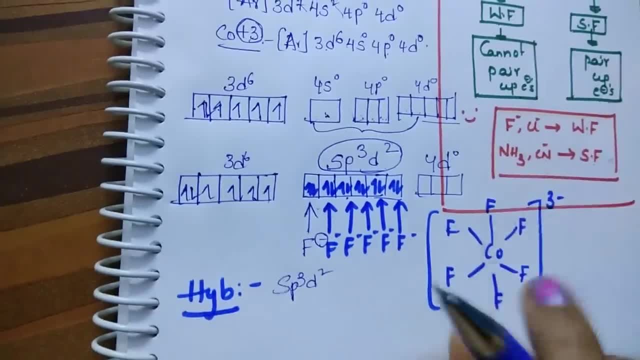 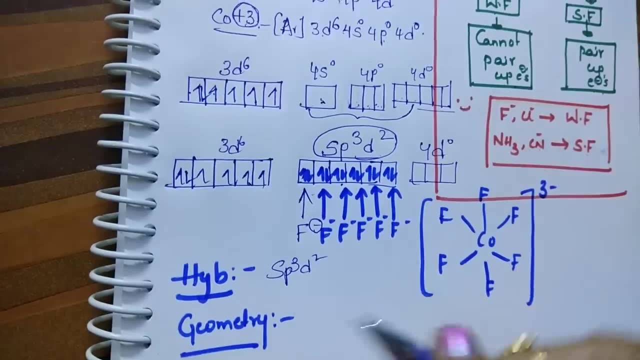 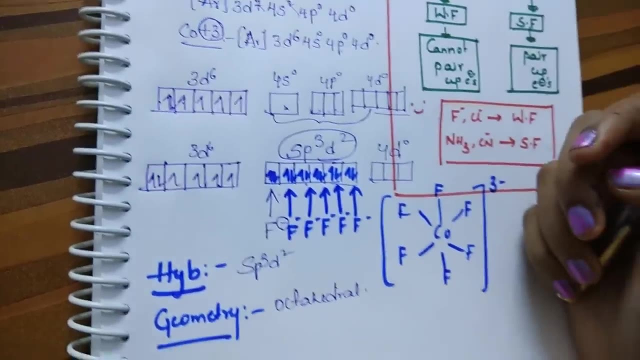 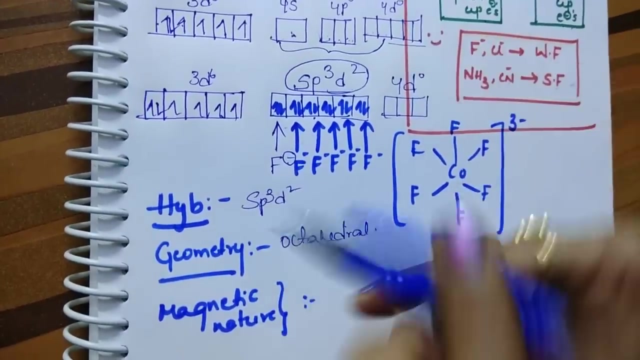 What is the hybridization? SP3D2.. And what is the geometry here? SP3D2- octahedral. And what is the magnetic nature Here? unpaired electrons are there. You should see only the metal atom electrons. 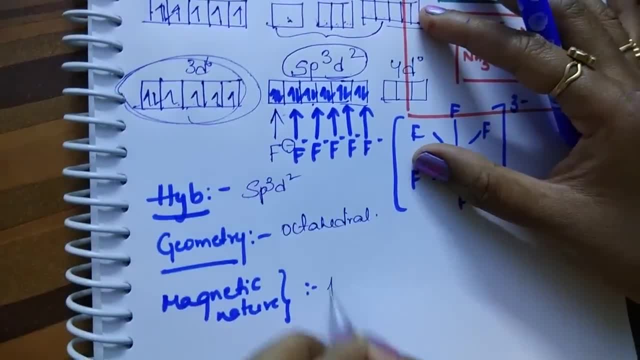 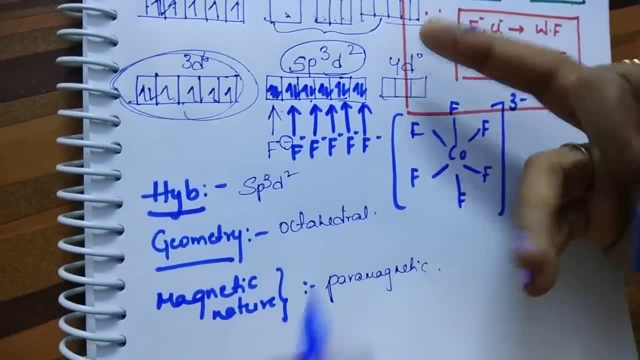 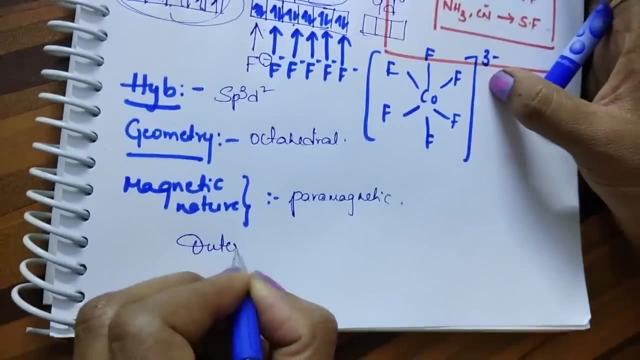 Here, unpaired electrons, single electrons are there. So it is paramagnetic in nature, Paramagnetic in nature And it used it's outer d-orbital, So it is an complex nature, is outer orbital, complex, Outer orbital complex. 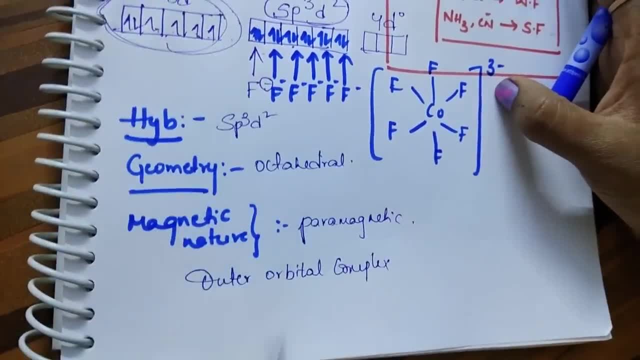 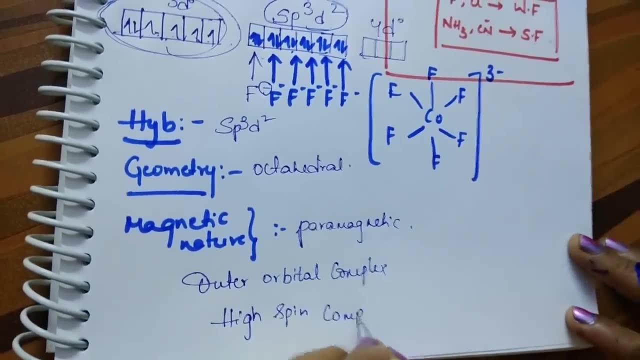 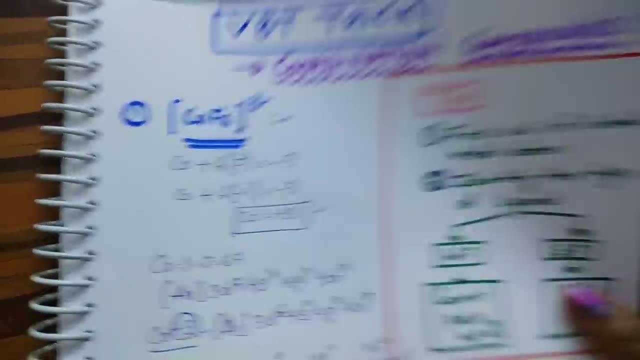 And here unpaired electrons are there. So it is a high spin complex, High spin complex. Right Now, you- I think I hope you understood this. Now what you do is just try for strong field again. 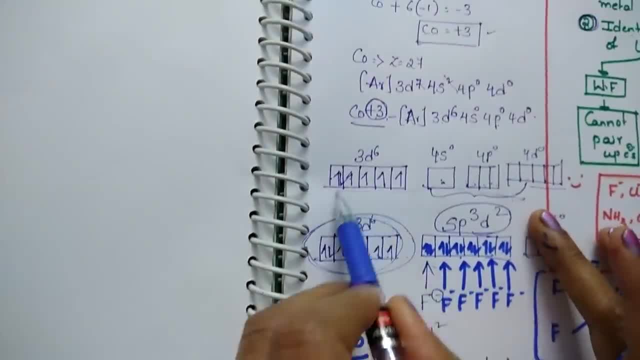 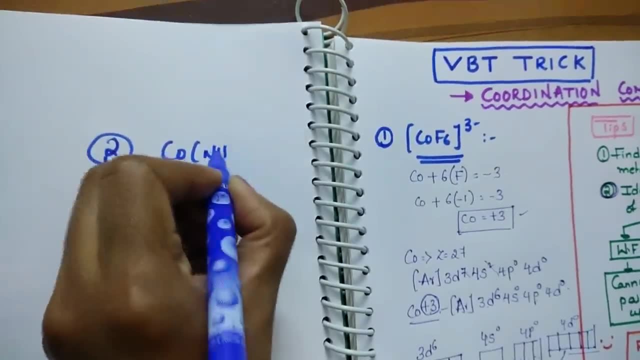 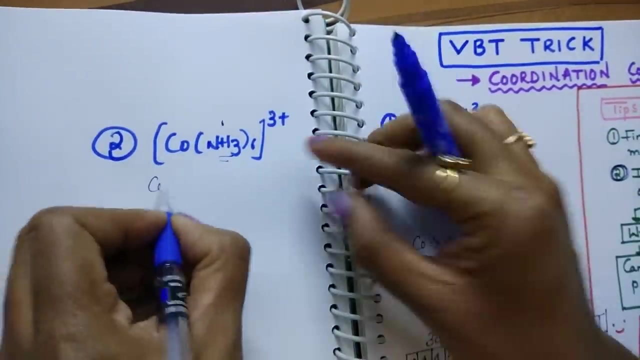 What I am telling you is up to here, it is same. Now, if suppose the complex is complex, is CO, NH3, 6, 3+, Then what you do here? Ammonia is a neutral ligand, So CO plus 6.. 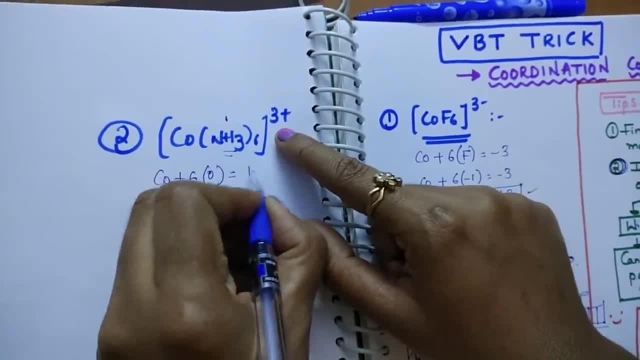 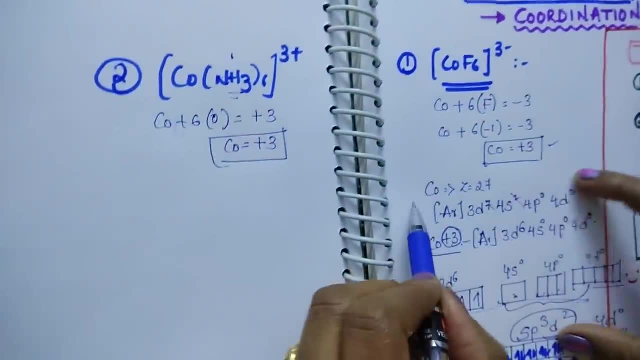 So CO plus 6 into its oxidation number is 0, which is equal to plus 3.. Then cobalt oxidation state here also plus 3. Then everything up to here it is same. After this fluoride ion, it is a weak field. 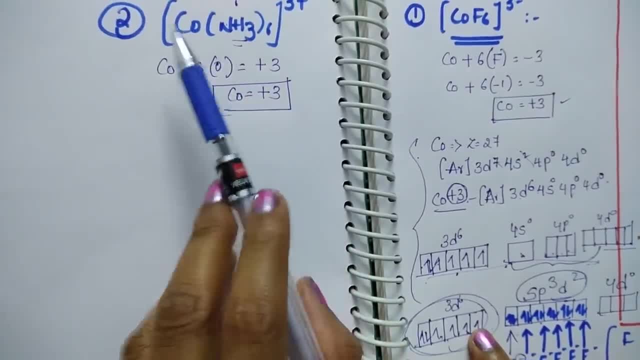 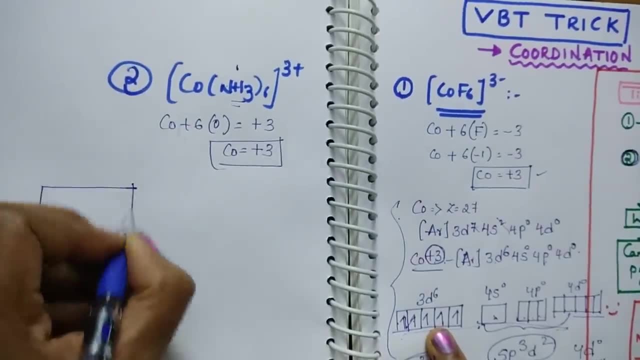 It cannot pair up the electrons. But ammonia is a strong field. again, Ammonia is a strong field. again, It pair up the electrons. So what happens here Here? 1, 2.. 3,, 4,, 5,, 6.. 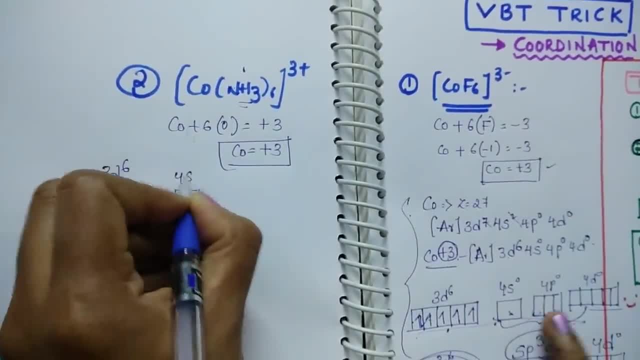 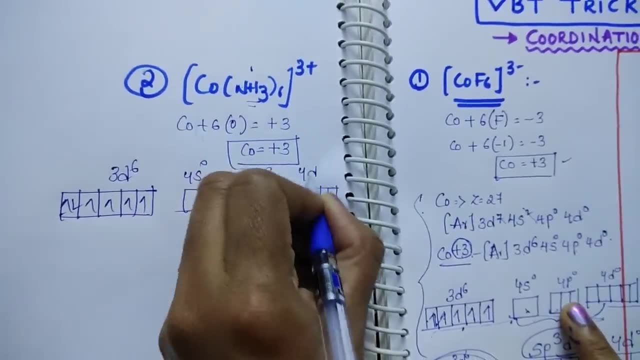 D how many electrons it has, 6. And 4s is empty, 4p also empty And 4d also there. That is also empty Right Now. ammonia is a strong field ligand. It pair up the electrons. Strong field. it pair up the electrons. This electron moves here, This electron moves here, So that 3,, 4, 5. Here 2 electrons, Here 2. Here 2. It makes this strong field again, makes 2 orbitals empty. 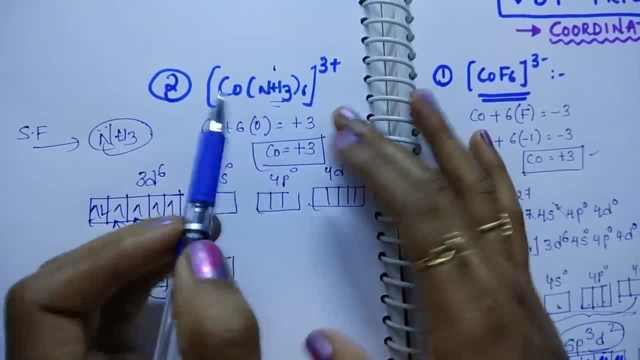 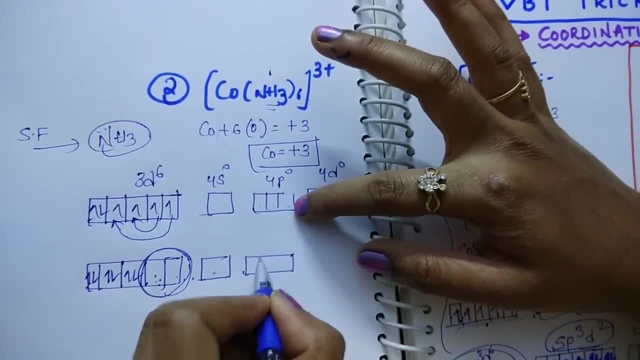 Then 1s Total how many it requires. 6 empty orbitals it requires. So 2, 1,, 2,, 3, and 4,, 5,, 6. Right, 6. How many it requires. 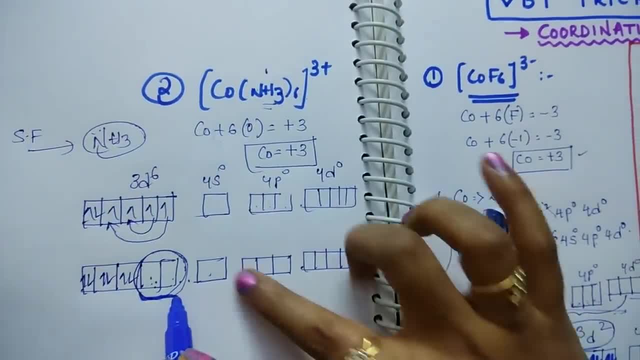 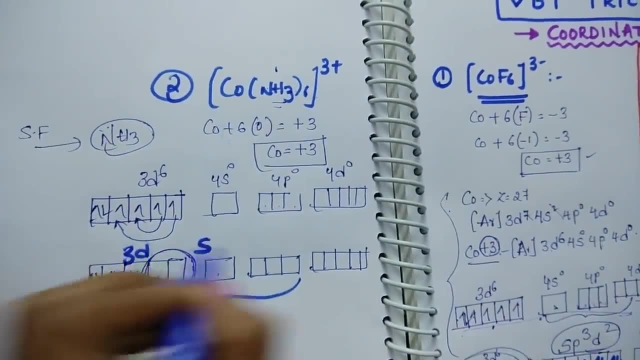 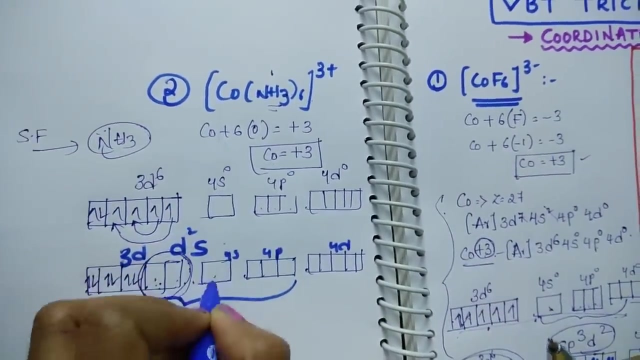 6. Right, These 2, this one total 6.. So 1s, How many This? These are 3d, This is 4s, 4p, 4d, Right. So 2ds d2, 1s 3ps. 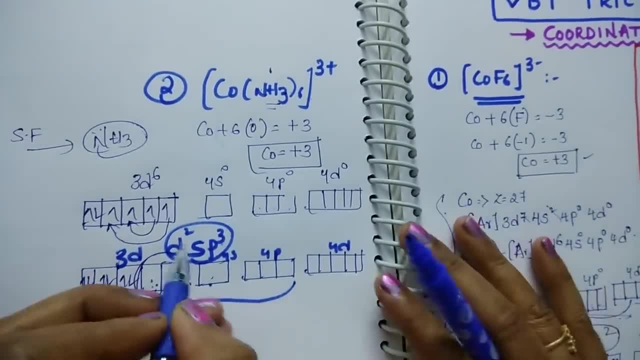 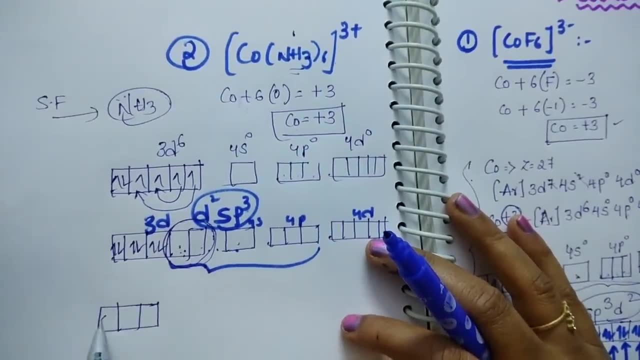 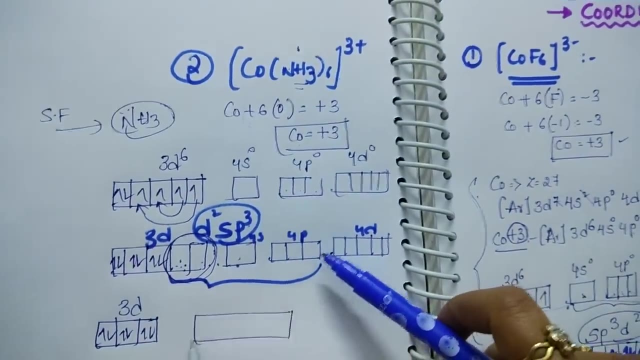 Total 6. 6. 6d2sp3 hybrid orbitals will be formed. These are metal electrons, 3d And 2d, 1s, 3ps. Total 6. 1,, 2,, 3,, 4,, 5.. 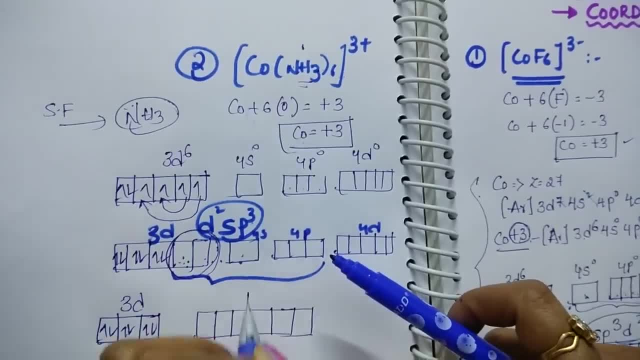 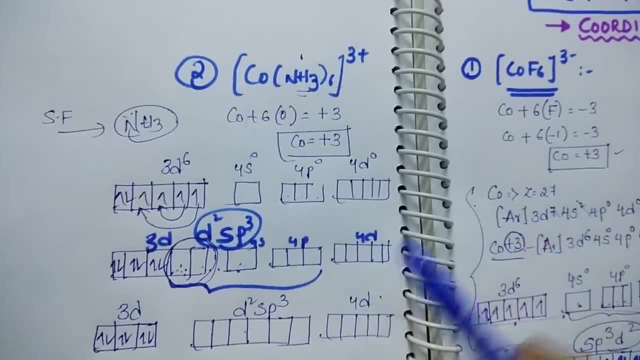 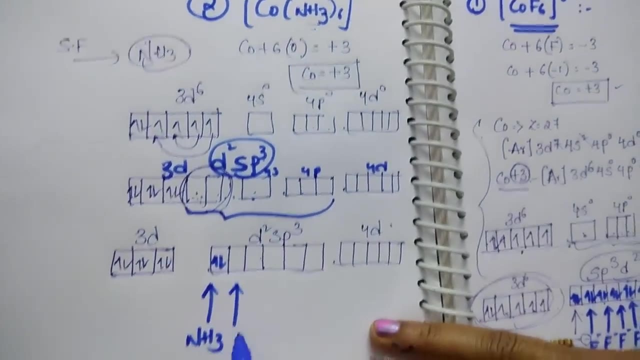 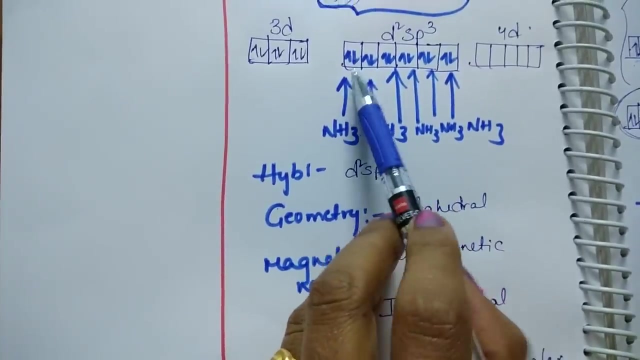 6d2sp3 hybrid orbitals And 4d will be empty as it is Now. each ammonia donate a pair of electrons to the central metal atom. Same way, Each ammonia donates a pair of electrons. 6 ammonia molecules donate pair of electrons each. 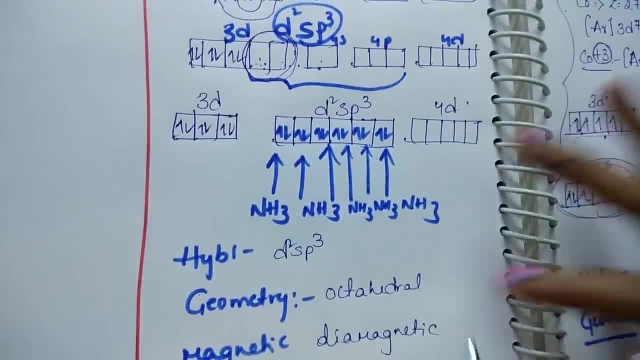 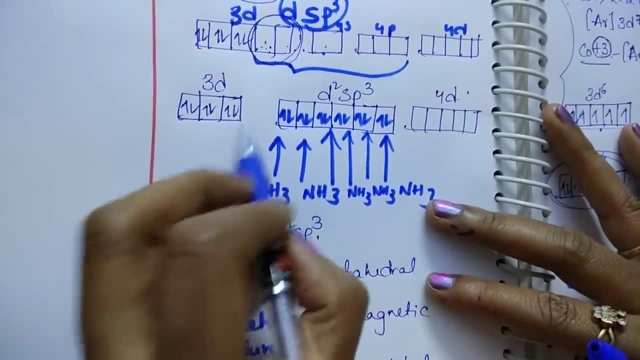 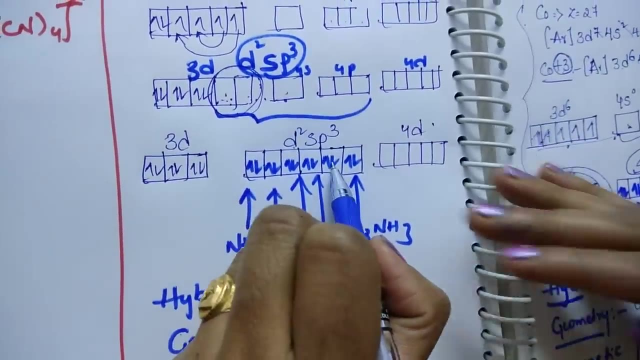 And it results in the formation of an octahedral complex. Here the hybridization is what students d2sp3.. Here there is no unpaired electrons in the central metal atom. It is diamagnetic in nature And it used inner d orbitals for the hybridization. 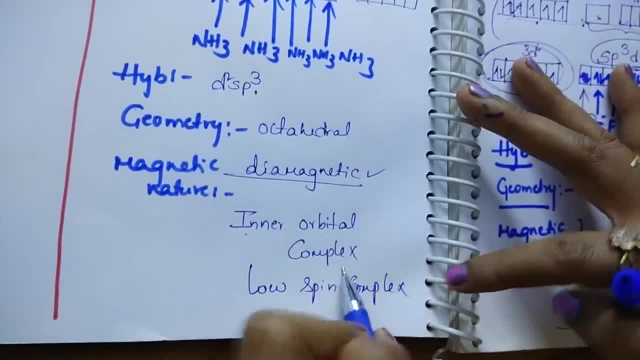 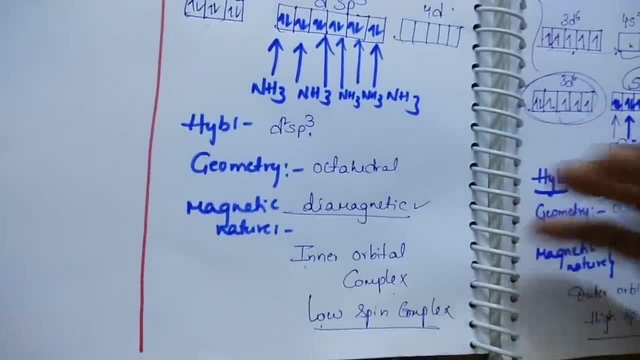 That's why it is inner orbital complex And there is no unpaired electrons. The spin is no spin here. Then it will be low spin complex. I hope you understood this, And what you do is Now. the term is over. 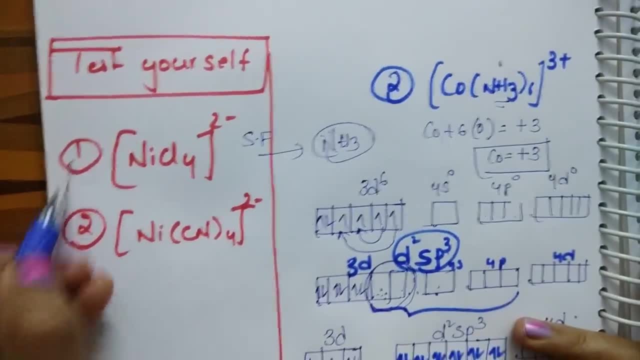 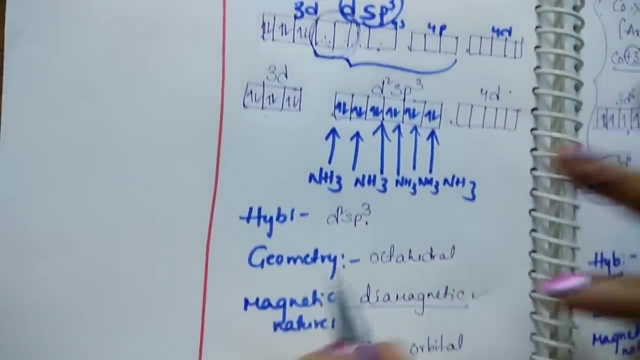 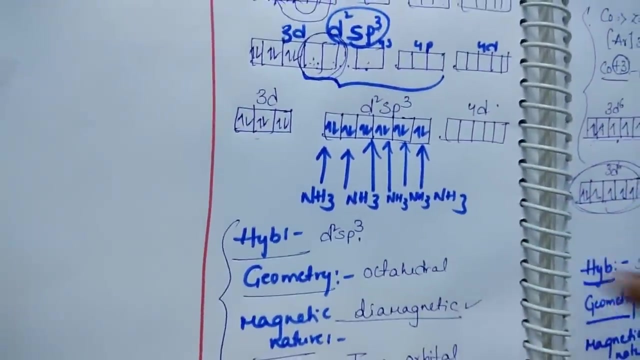 Now the time for test yourself These two examples. Try it. Try using this method, Easy way. Just, you find hybridization, geometry and magnetic nature And comment me your answer. Whether you are getting the answer or not, See one time I am revising. 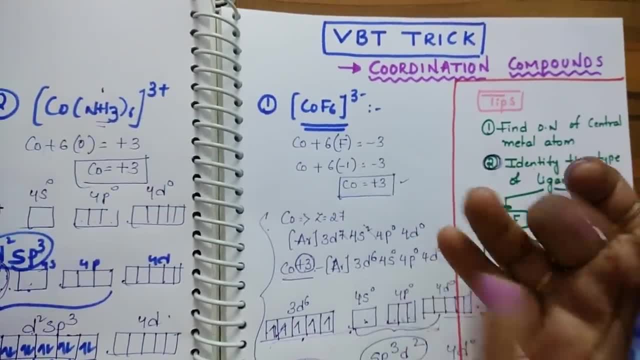 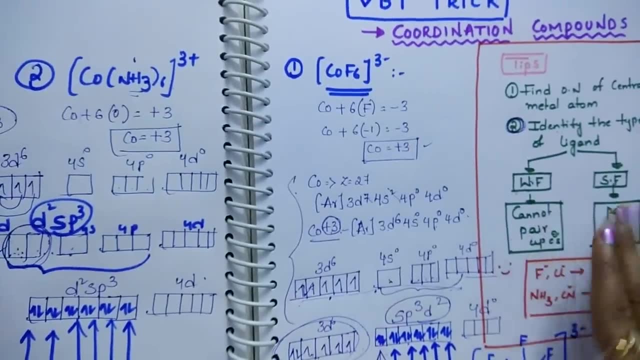 What you do is Just find the oxidation number And write the electronic configuration, Identify whether it is a strong field or weak field. again, If strong field, it will pair up, If weak field, it cannot pair up. Thanks for watching my video.